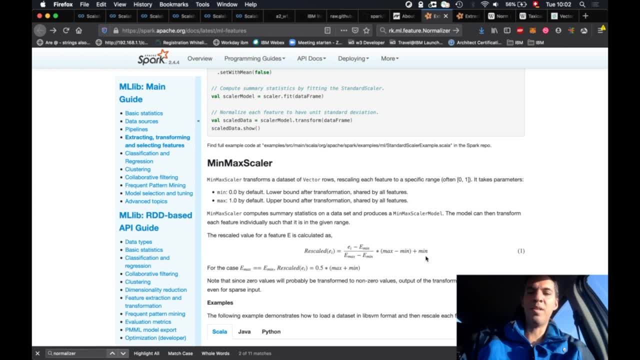 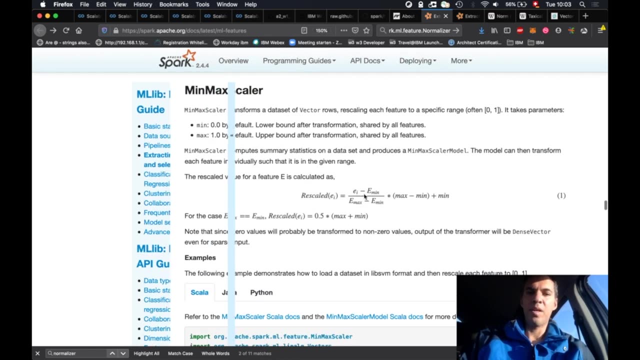 Plus min, that's still 1, and if you multiply something by 1, you get basically this formula here and this formula here- let's increase the size a bit- not working. So this formula here is basically the same we have just seen, okay. 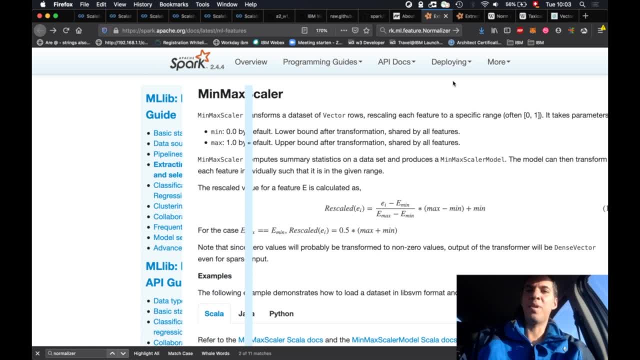 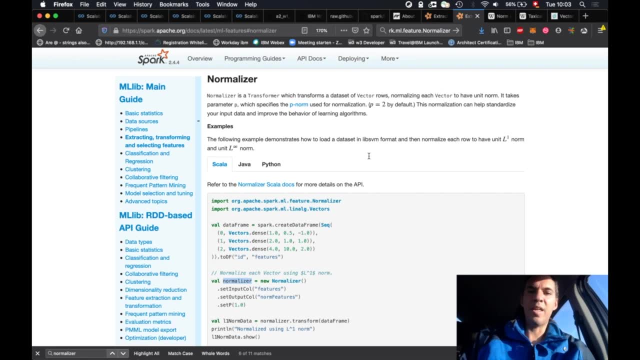 So now let's have a look at the normalization function and if we have a look at the Spark documentation, Then it says it uses the so-called p-norm. okay, So if we have and it uses, p equals 2 by default. so let's keep that in mind. 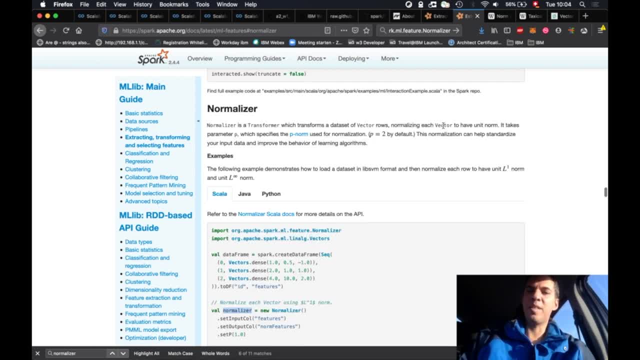 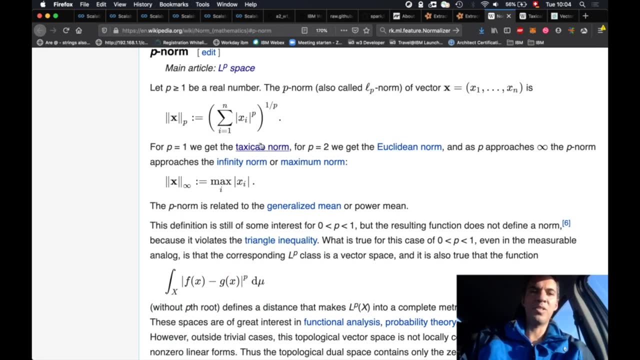 So you have a vector as the input and it computes the norm of the vector. okay, keep that in mind, that you have a vector. So if we have a look at the definition here, this is the vector and those double bars are the symbol for the p-norm and p stands for the parameter p. 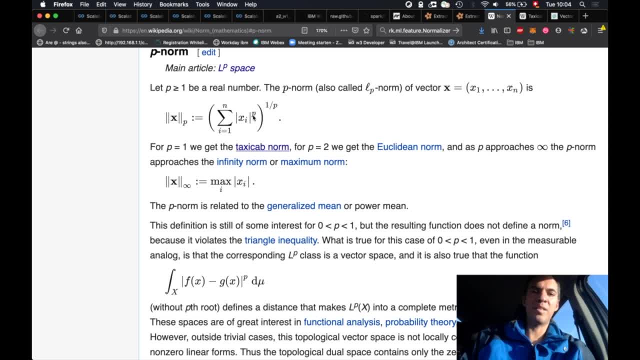 And here you basically just take the value or the element of each vector. you use the exponent p and then you sum those values up, and later you just take the use the exponent 1 over p. okay, So if you have p equals 2, you get the Euclidean distance. 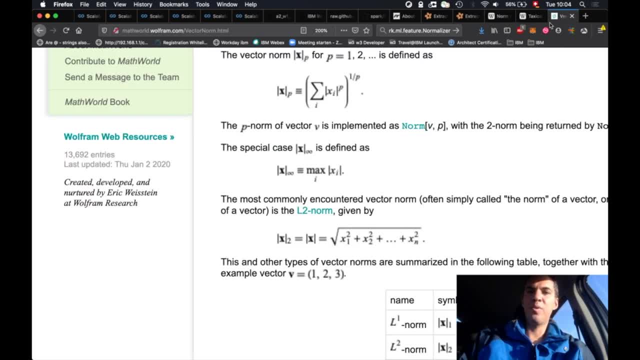 Let me show that to you. So let's consider p equals 2, that means you square each element of the vector and later on you take the square root, because taking using the exponent 1 over 2 is basically the square root. So you see that here you have here x1 squared plus x2 squared, and so on, and then you take: 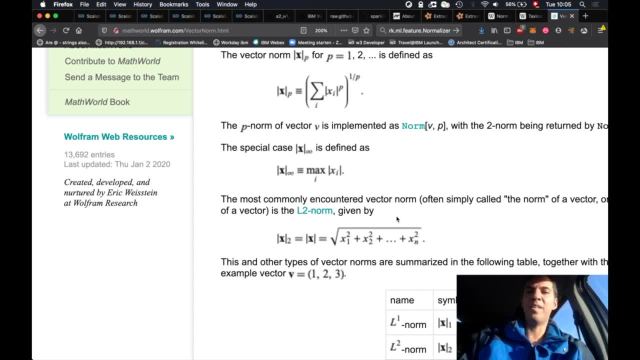 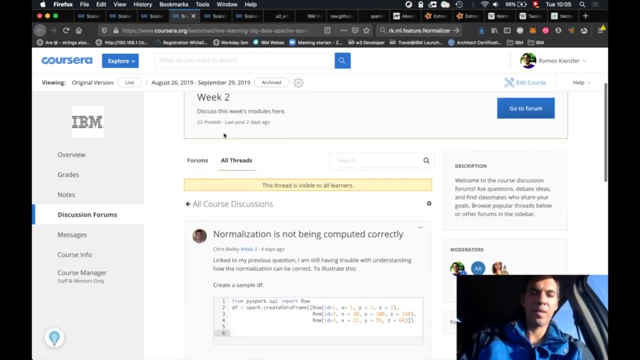 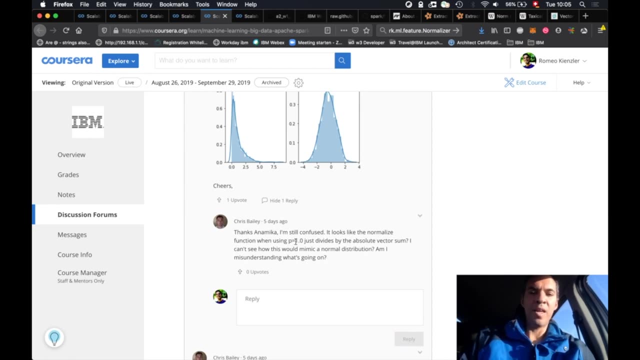 the square root of everything, okay, And that's also defined as the Euclidean distance. And now, since you asked: Okay, Where was the question? ah, since you asked here. So you are confused because you used p1 and then you say it just divides by the absolute. 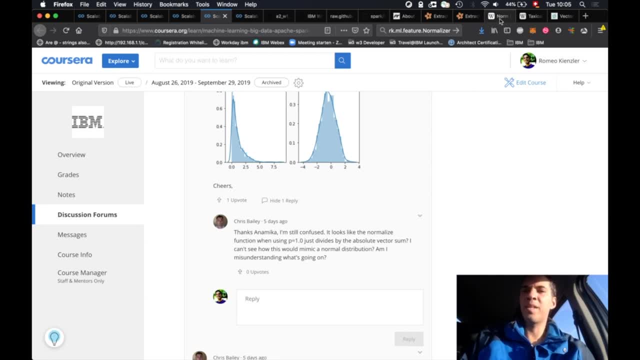 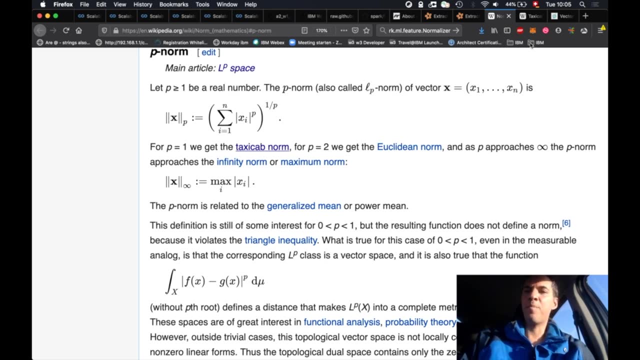 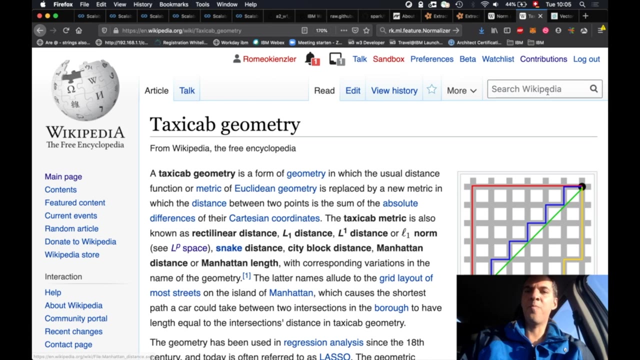 vector sum. So this is not 100% correct, because if you use p equals 1, you get the so-called Manhattan or taxicab norm And that's basically just subtraction. It's just summing up all individual values of the vector, which is pretty clear if you.